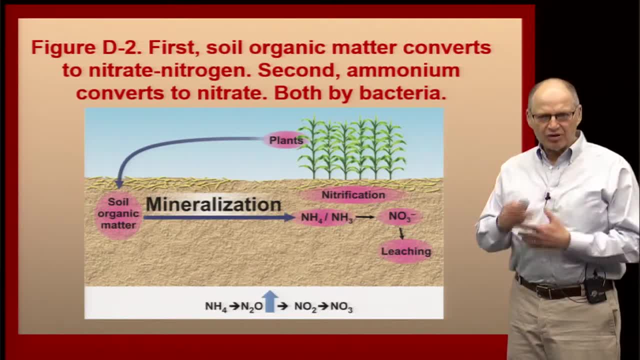 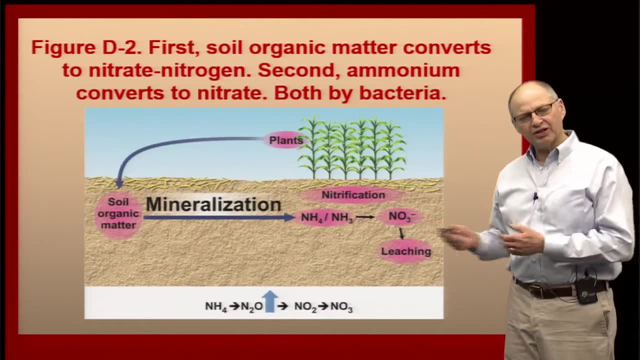 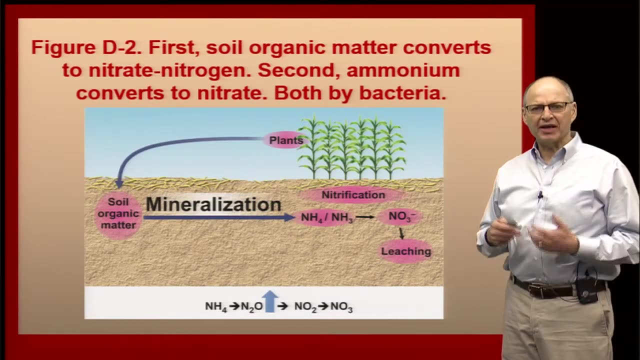 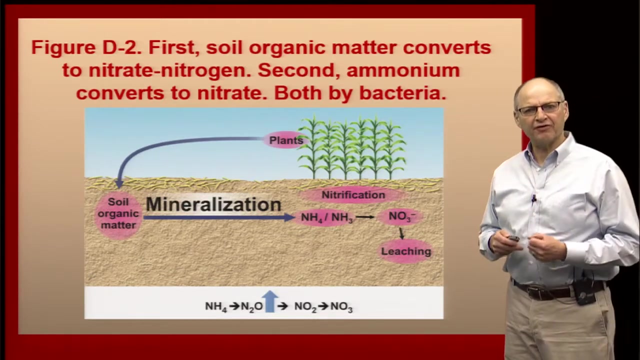 important thing is to know that these processes are going on and what are the conditions when they happen. the most so for mineralization, which is the transference of nitrate or nitrogen from, say, organic material, whether it's manure or soil, organic matter or compote or just dead plant material. the nitrogen has to be split off from the 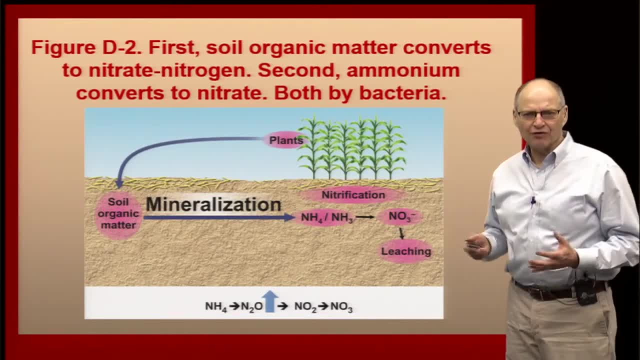 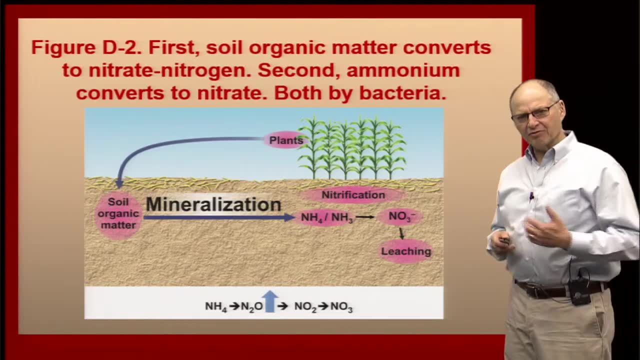 organic source, and when it's split off, it's in an NH form- whether it's ammonium or ammonia depends on certain conditions. and so that's the process of mineralization, basically mineralizing going to a chemical from an source. the next step is nitrification, and that's when it goes from the 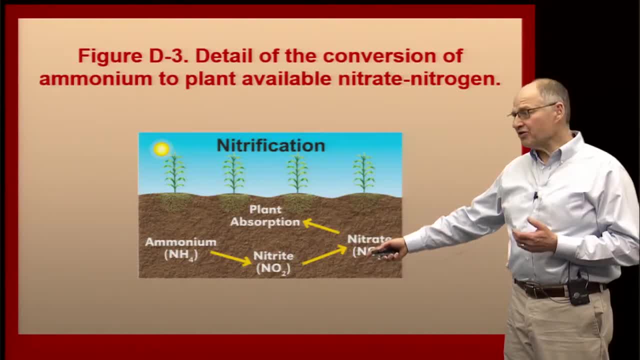 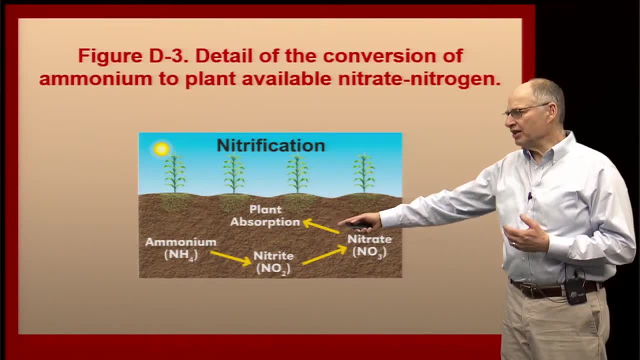 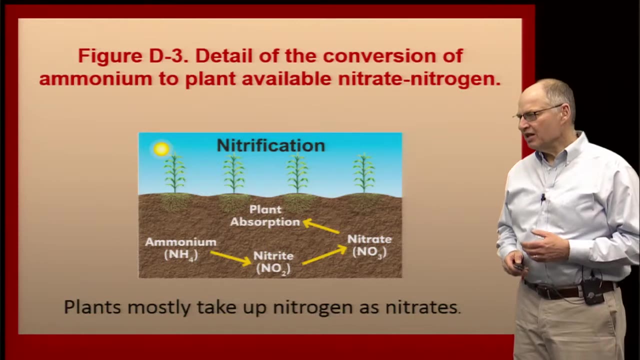 ammonium source to nitrite doesn't stay in nitrite very long. then it becomes nitrate and although plants can take up ammonium as well as nitrite, most of the end going into the plant is in nitrate- nitrate, excuse me. so that's what we. 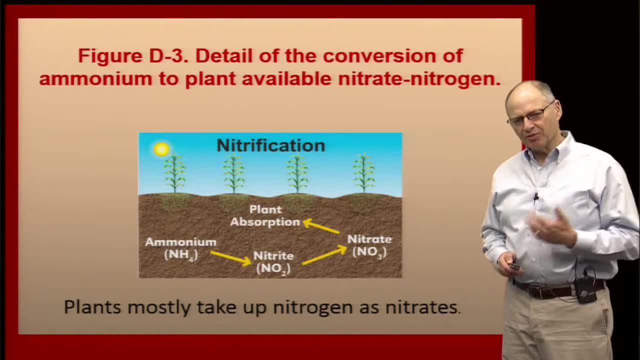 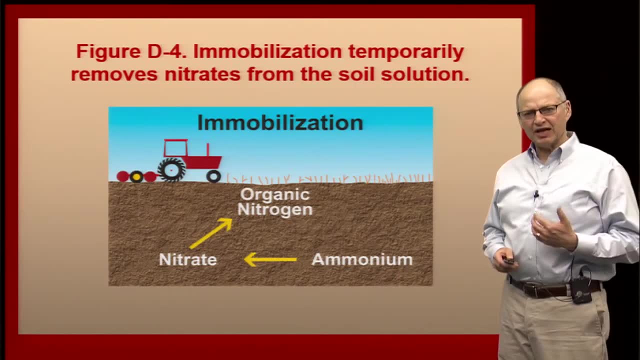 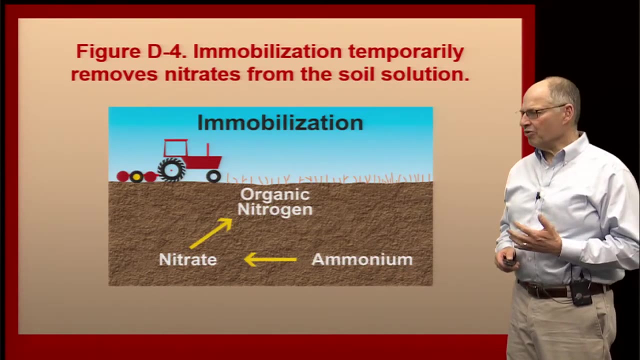 really want to keep track of as the nitrates, because the ammonium is not going into the plants very well now. once it gets into nitrate, that doesn't mean it's going to go right into the plants. conditions can arise where it can leach. 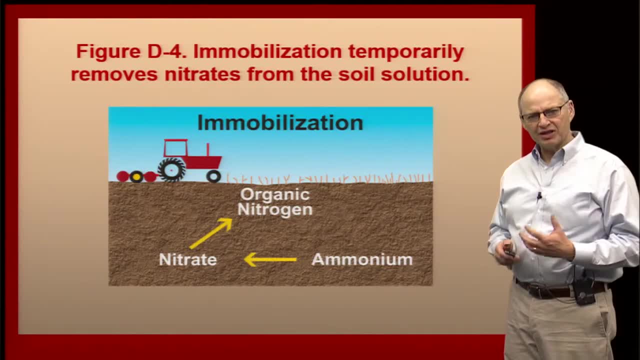 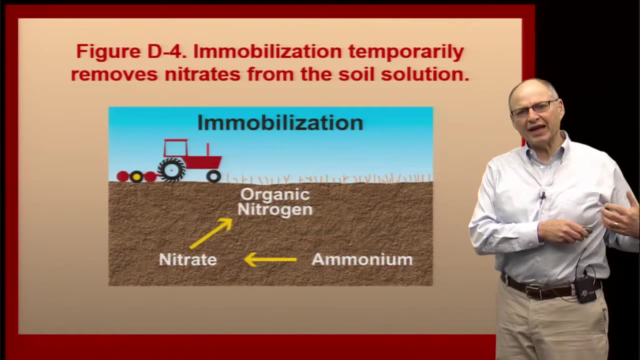 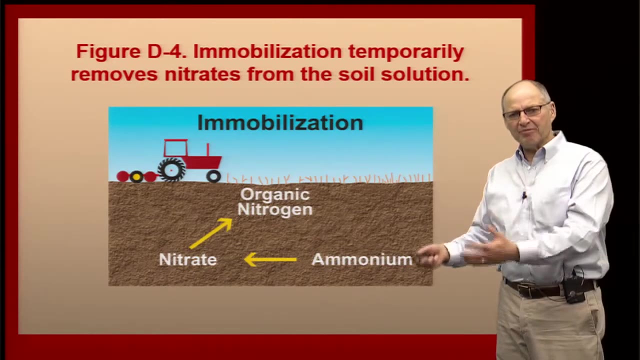 but in this case we're talking about immobilization, which is where it goes. that's the opposite of mineralization. the mineralization move the the organic material into the ammonia form, and here we're taking the nitrate and putting it back into the organic form. and that happens when their microbes in 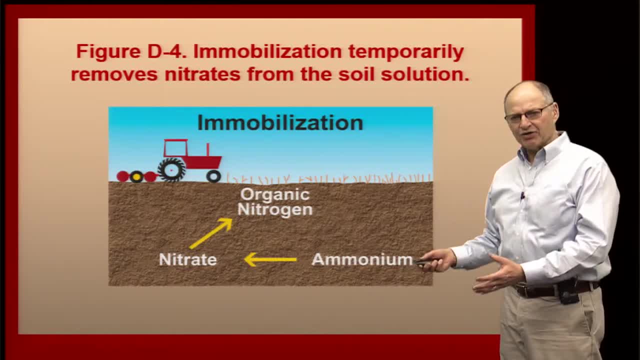 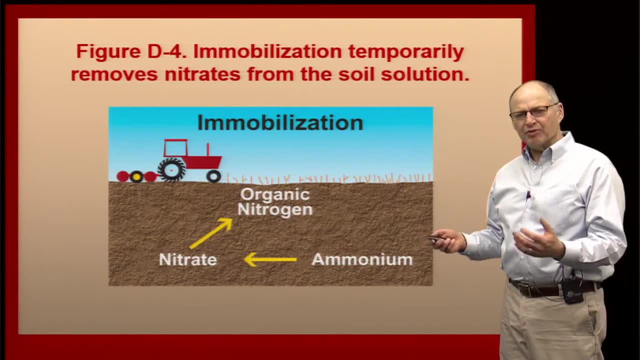 the soil and there's a lot of carbon, and the microbes use nitrate as a food source of it, helps them grow, and so that's this will happen when you might have a lot of corn residue or a lot of wheat stubble and not a lot of nitrogen. 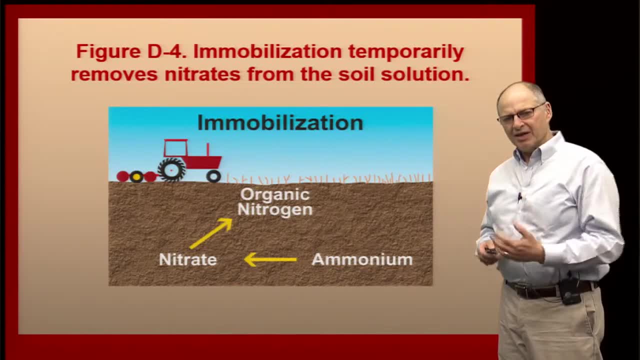 there that nitrogen is put into the organic matter and that makes conditions where the nitrates are very low in the soil and your crop can turn yellow for a while. eventually those organ micro organisms will die and they will release the N again, but for a while it's immobilized. 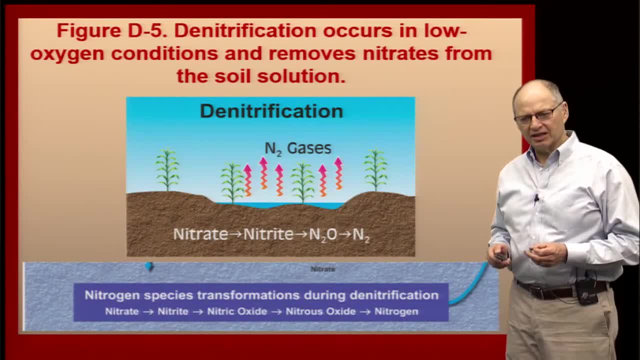 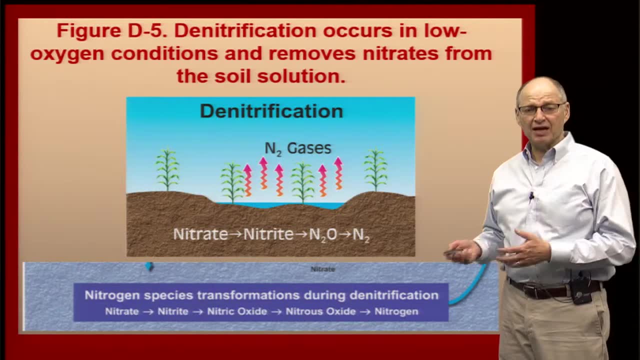 one condition called denitrification is probably a condition that doesn't happen to be a very bad condition is a condition called dehydration or nitrification, which is probably a condition that doesn't happen that much in Nebraska, especially during our drier periods, but we have times in the spring. 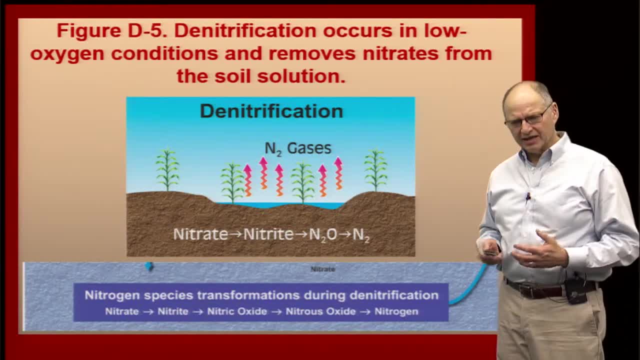 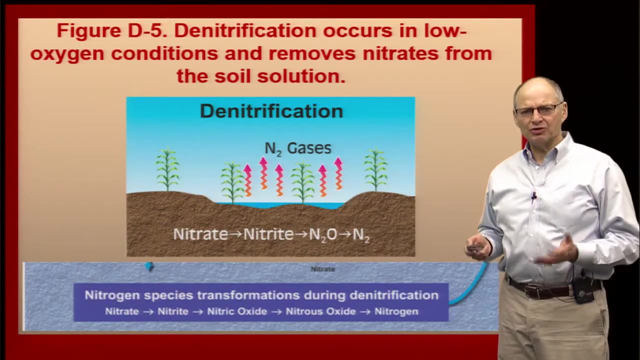 and there are places in the landscape where water will collect. and whenever we have water sitting saturated soils for more than two or three days, we create conditions that are called anaerobic conditions, which means there's no oxygen, and then microbes use the nitrate. 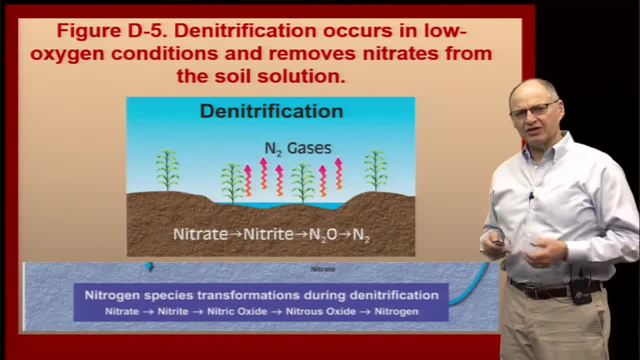 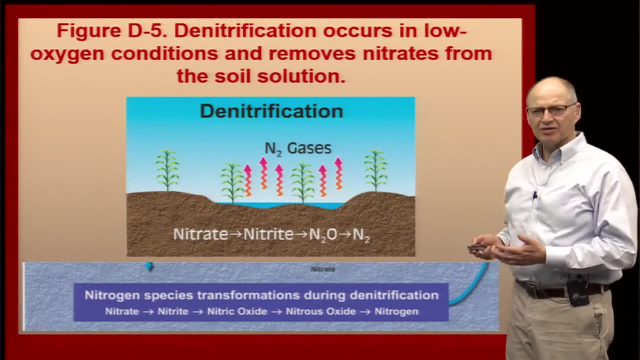 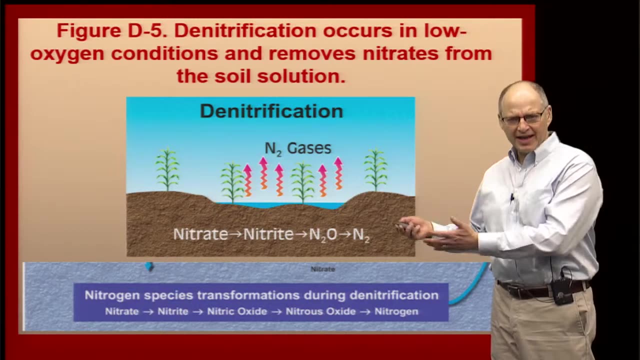 as an energy source and they break the nitrate down ends up going into the atmosphere as N2.. So, even though this isn't a major loss mechanism for us, when you go farther to the east of the United States, into Illinois, Indiana, Pennsylvania, where they have a lot wetter springs this: 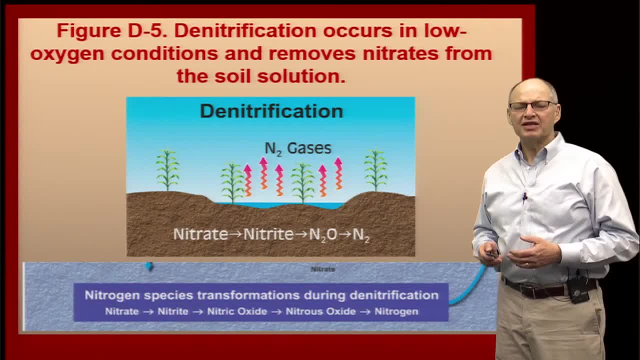 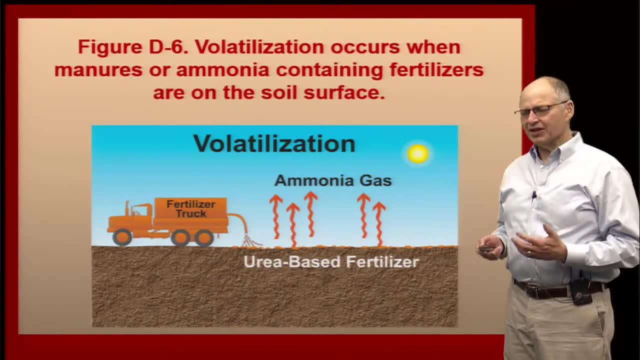 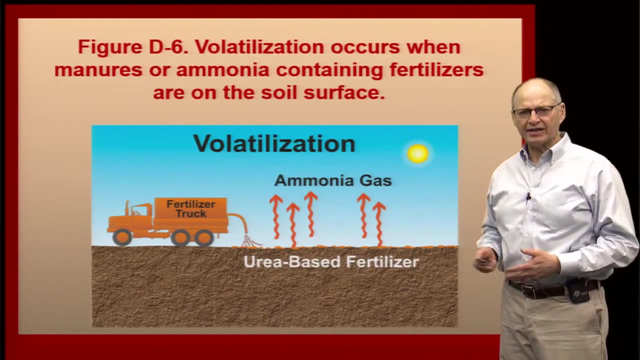 denitrification is a bigger problem, But there are situations in our landscape where this might occur in some years If we step back and think about putting fertilizer on our soil and not incorporating it, which sometimes is a good practice, and many people are in no-till and they do have to just put the 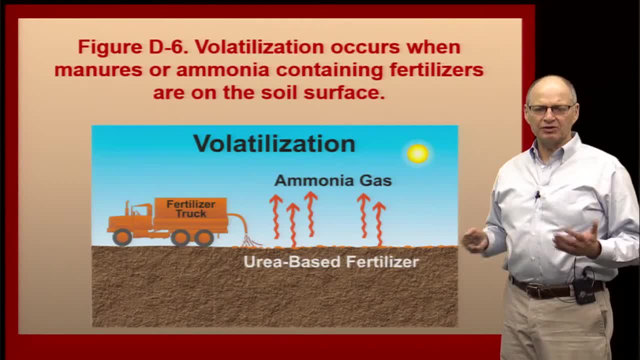 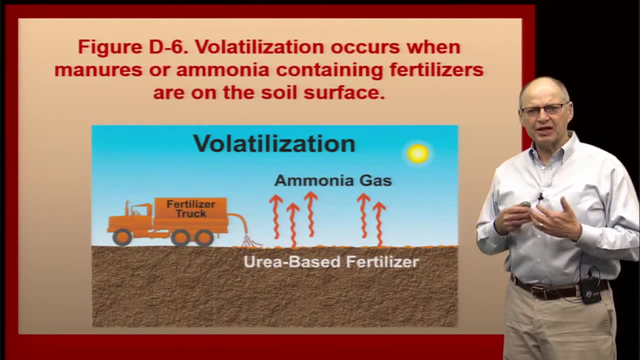 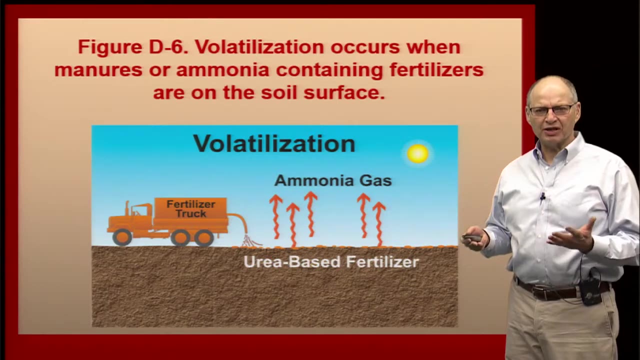 nitrogen on the surface. there are conditions where we will lose nitrogen to the atmosphere. What happens is the ammonia urea breaks down, and when it breaks down it's called hydrolysis, and that hydrolysis produces free radicals. If the urea is in the soil, if it's incorporated in the soil, then that ammonia gas will attach. 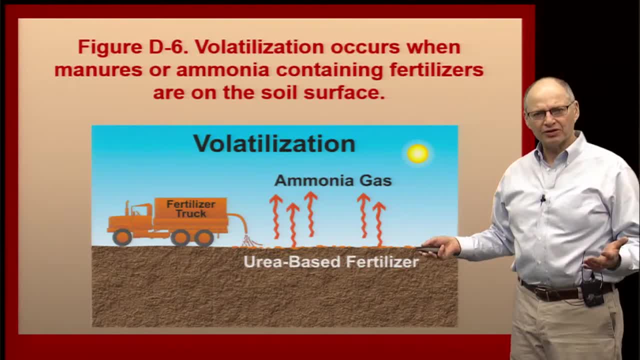 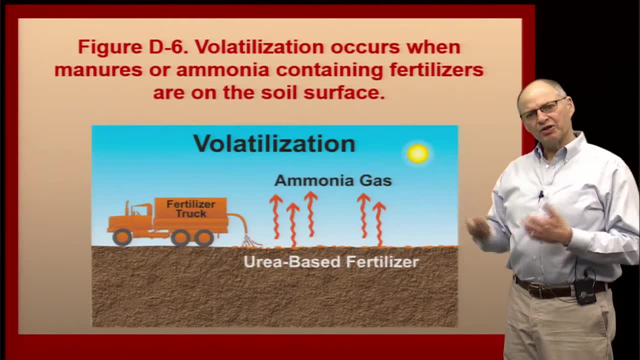 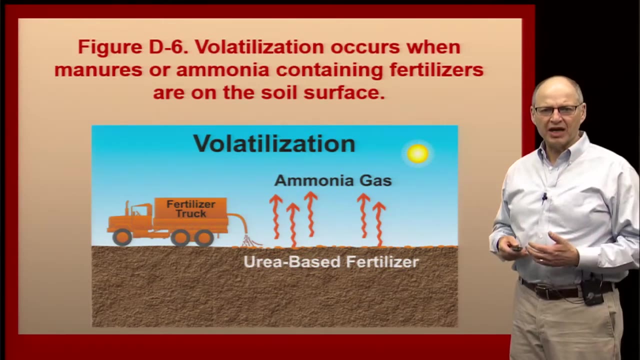 to clay particles- organic matter particles- it could go into the water solution, But if it's sitting on the surface of the soil, that ammonia gas will go into the atmosphere. So that's something we have to watch for. If we get rain- about a half inch of rain after we apply urea or UAN, that's enough. 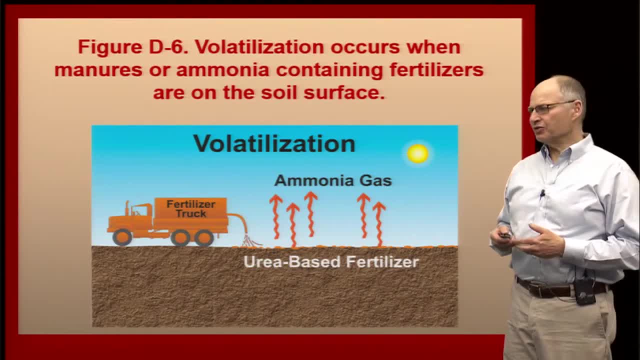 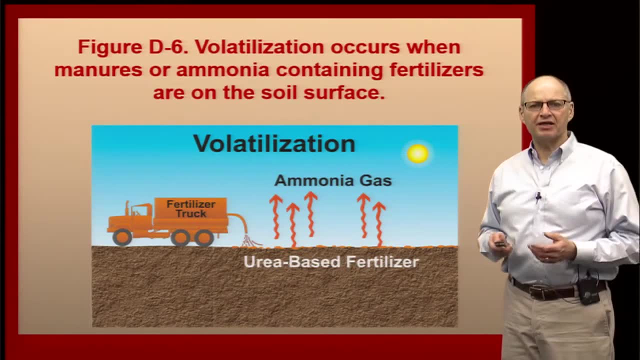 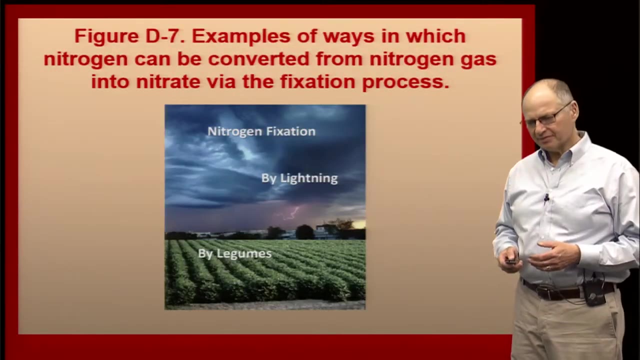 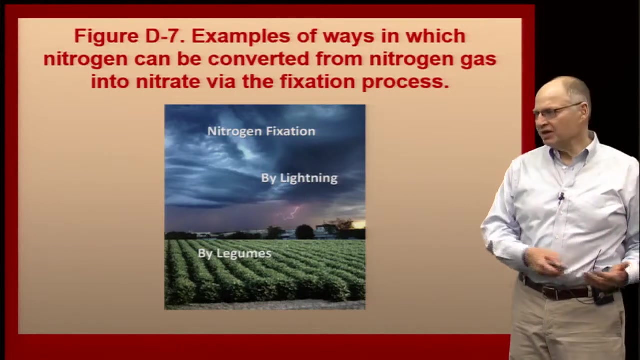 water to move the material into the soil Or you can irrigate it on. We do also have some nitrogen additives called urease inhibitors that will protect from this hydrolysis for 10 days to two weeks, Kind of as an aside. there are ways that we can get nitrogen going back into the soil. 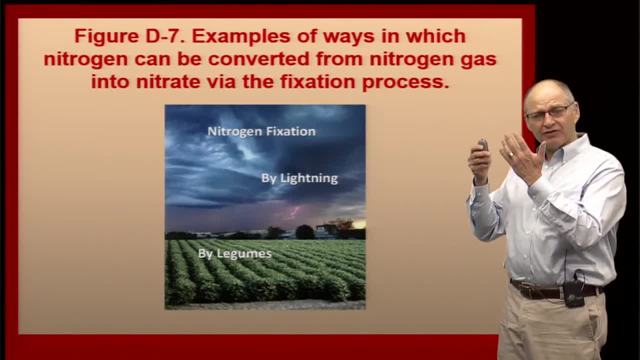 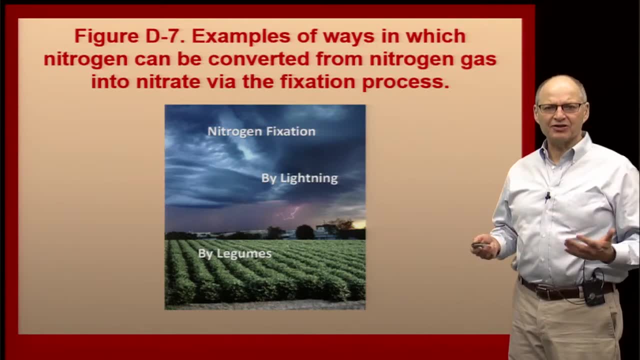 Everything I've talked about so far has been either losses to the atmosphere or, you know, water. We've talked about putting the nitrogen in a condition where it might leach, But over time- and this is how the nitrogen, most of our nitrogen, got into the prairie. to begin with was through nitrogen fixation by lightning. It takes a lot of energy to convert the N2 gas into ammonia because of the chemistry of it, But when you get a big lightning it has a high charge and it does put a hydrogen bond. 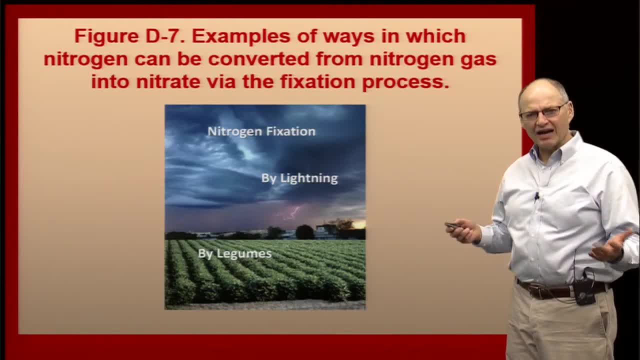 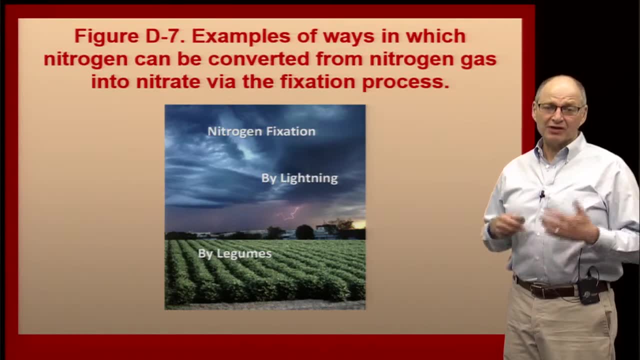 into that nitrogen. So even if we might gain five, six, seven pounds a year per acre, you know that's not a lot of N You can't grow a crop on it. But if you have 10,000 years of getting seven pounds a year, that slowly gives nitrogen. 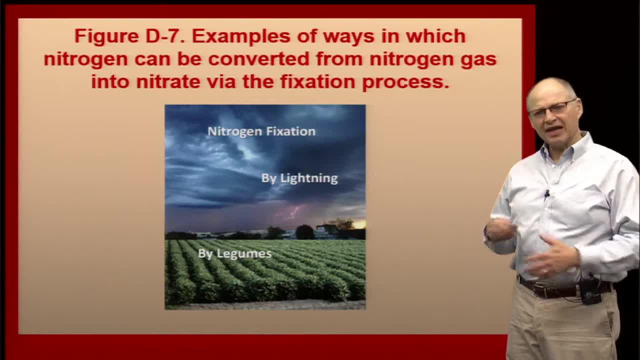 to our soil And back when there was prairie, that grass would use it and the grass would die, And then the next year it would break down and new grass would come, And that's how come we ended up with 18 inches of topsoil. 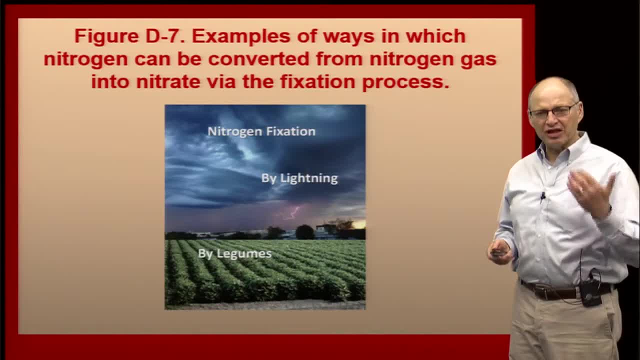 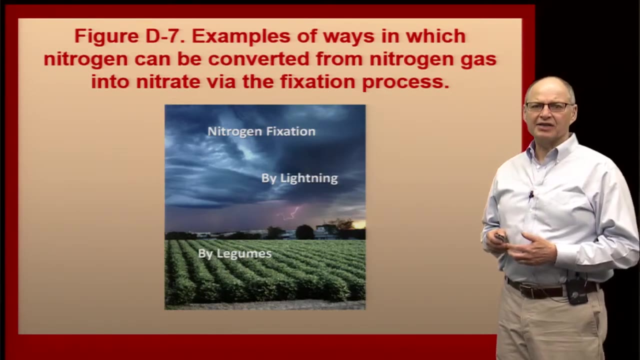 Now in our agriculture we have legumes that, through microbial symbiosis bacteria in the roots- do the same thing as the lightning for the most part, And they can fix- alfalfa can fix- 250 pounds of N a year, So that's another way we can get some nitrogen back from the atmosphere into the soil. 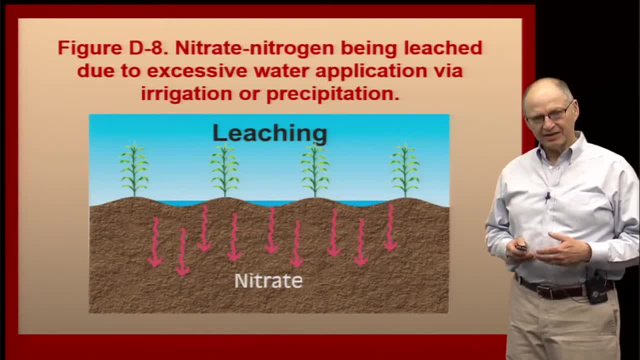 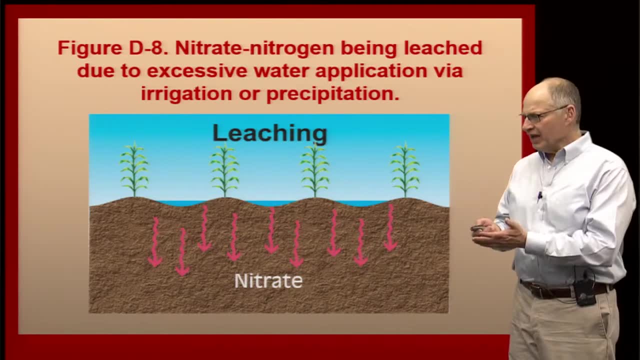 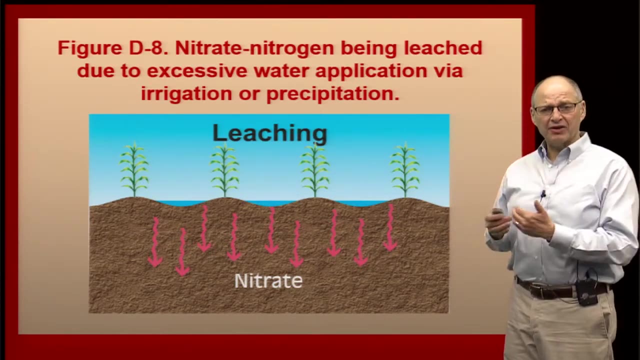 Again, that's part of the nitrogen cycle. The next loss Mechanism is leaching, And we get leaching when you have nitrate. Ammonium doesn't leach. for the most part It attaches to the soil, either the organic matter or the clays. 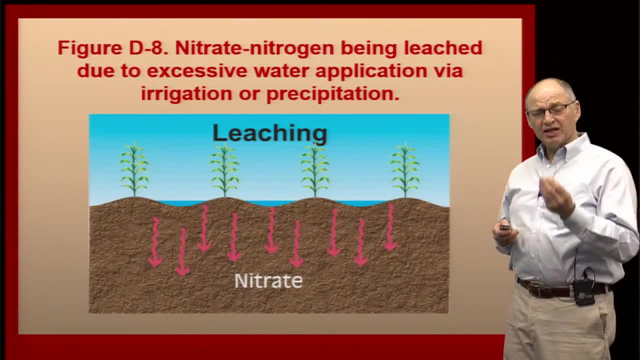 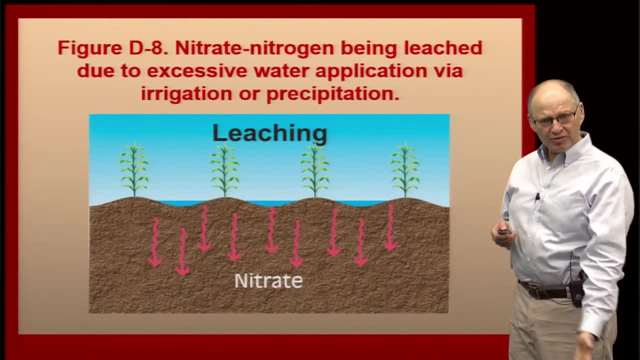 But the nitrate will leach because it's water soluble. It's in the soil water And if you have drainage, if you irrigate too much and the water moves, if you have a big rainstorm and the water moves, that nitrate is soluble and it moves with the soil. 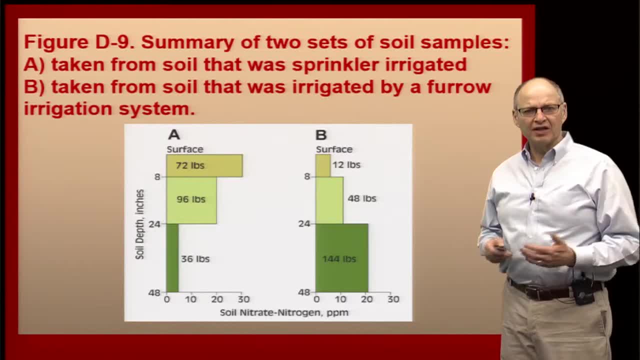 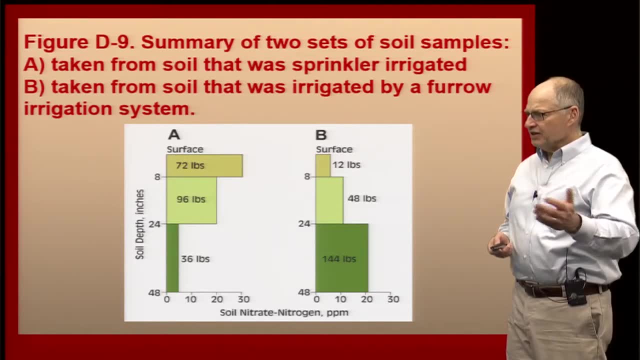 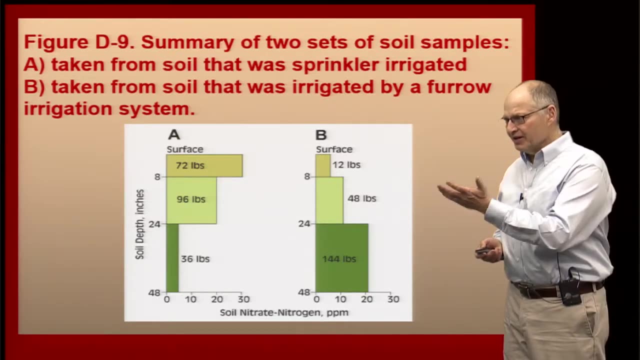 water. Here is an example of two different situations, different irrigation situations: The surface irrigation on the left and the- or, excuse me, the sprinkler irrigation on the left and the furrow irrigation on the right And the sprinkler irrigation where they can control the water better and they don't have 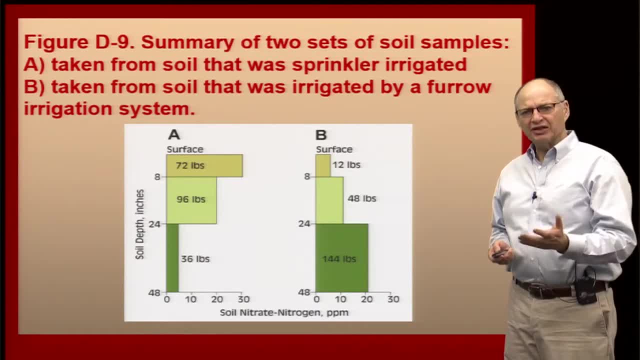 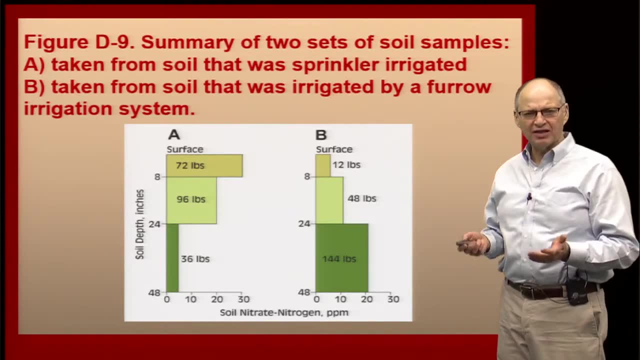 high levels of water going on at any one time. the soil nitrates at the end of the season are concentrated in the above. Both these figures have the same total pounds of nitrogen in the top 48 inches. But where there was furrow irrigation and there was a lot of water going through, it's 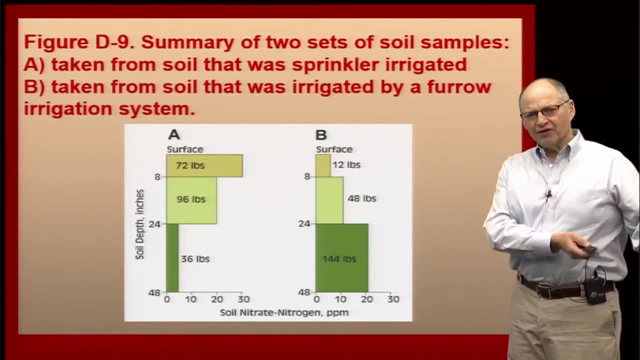 not as well controlled. It's not as uniform. Furrow irrigation starts near where the water comes out. compared to where it goes to the end of the field, It's not the same amount of water going in. So where there's a lot of water going through near that initial pipe, you might be leaching. 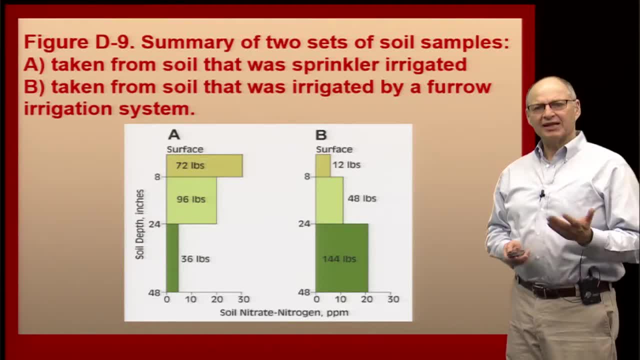 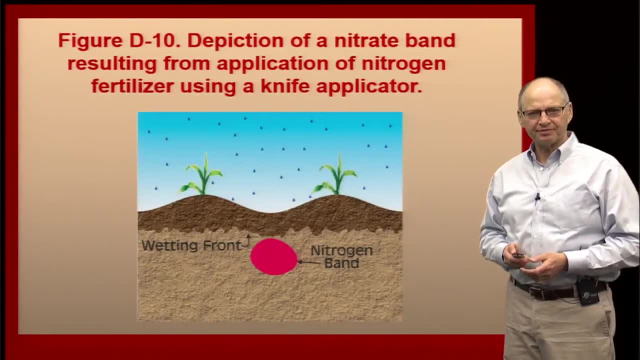 some N, And once you get the N down below 4.5, you're good to go. If you get the N down below 4.5 feet, most crops can't take it up And so it's lost, and could be could get to the groundwater. 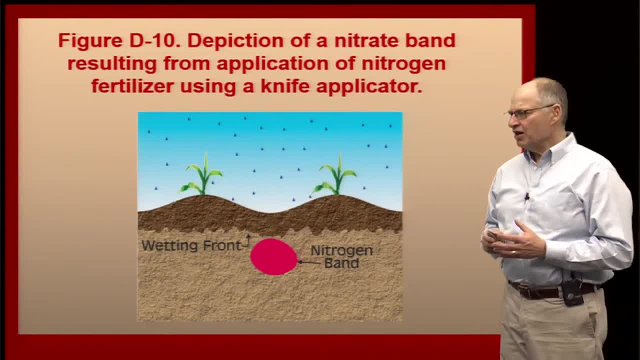 So if we want to visualize how nitrogen might move in the soil, we have here the idea of a band, whether it's an anhydrous band or a UAN band. Now, if it's a UAN band, it's not going to be the same material as an anhydrous, because 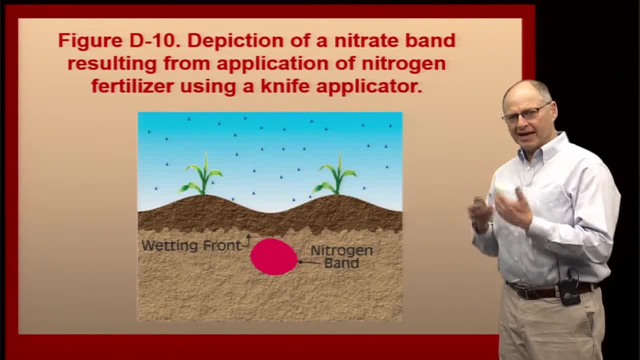 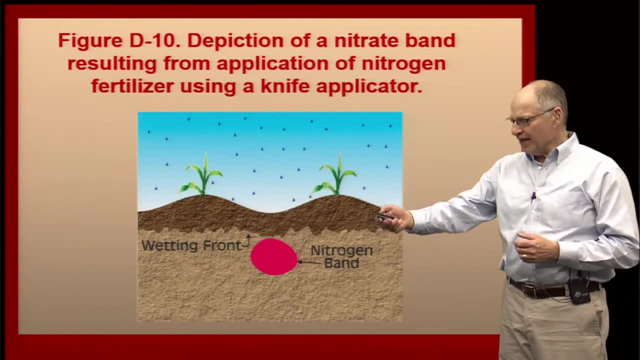 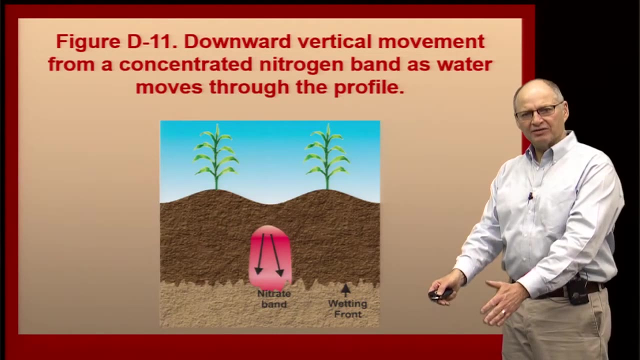 UAN has ammonium nitrate as well as urea, And anhydrous is just, It's just ammonium. But you put that in there and then, here you see, the darker part is the wet And then, as it, as the water goes through the profile, the nitrogen goes down with it. 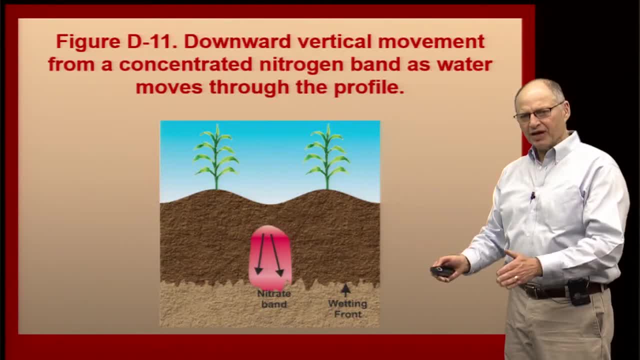 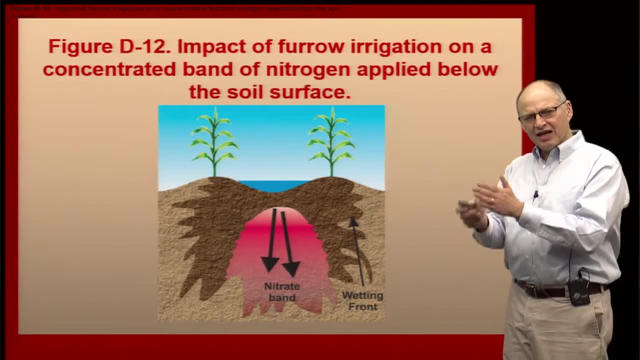 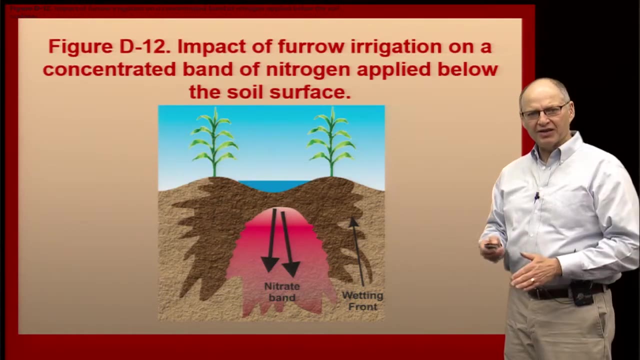 And it stays. it spreads out a little bit, but it doesn't spread out that much. If you have a furrow irrigation where you're just irrigating through the furrow and your band is below it, It's going to spread out more because the water is spreading out to dry areas. 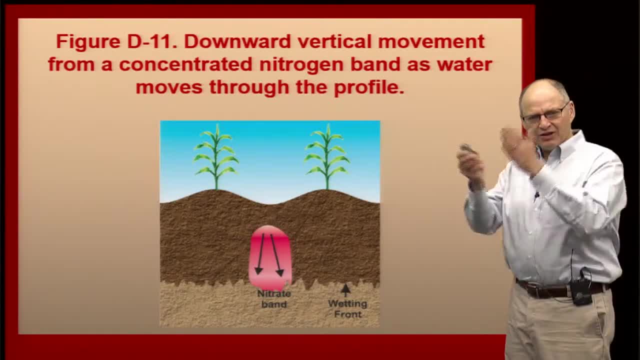 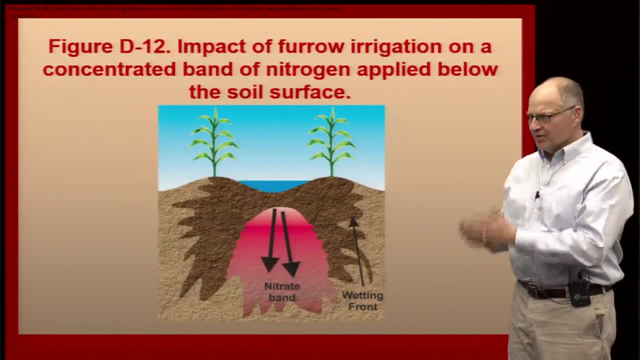 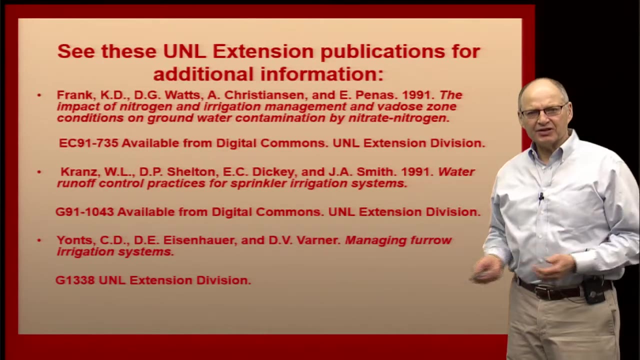 If we look at the previous slide, where everything is wet, then you don't get that spreading out because there's water across the whole surface there, But here, because it's coming down and out, we get a little bit bigger spread. So there's a lot more that we can say about nitrogen and how it moves through the soil. 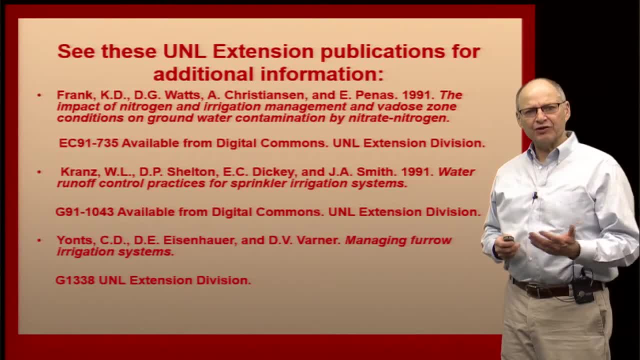 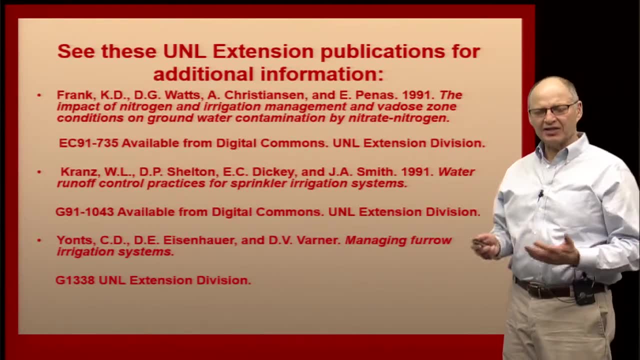 but we're going to end here. Okay, Just leave you with a few of these extension publications. Some of these are not currently in our extension publications site, but in the digital commons, which you can just type in your browser digital commons, you can find some of these publications.